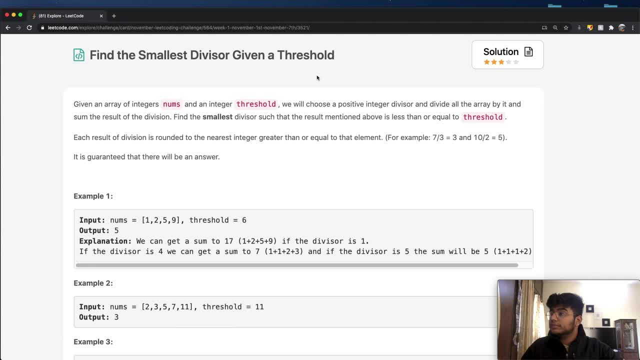 threshold, We will choose a positive integer divisor and divide all the array by it and sum the result of the division. Alright, so basically, we're going to be choosing a number and this number is going to be our divisor. So what we're going to do is- let's say this over here- is our 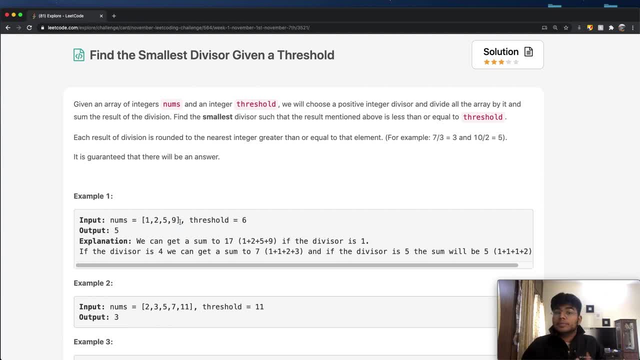 integer nums and let's say we have chosen a number three, So three would be considered our divisor. Now we're going to divide each of the numbers by three and then we're going to sum it up: Okay, and that's what we want to do. And now, after doing that, what we're going to do is we're going to 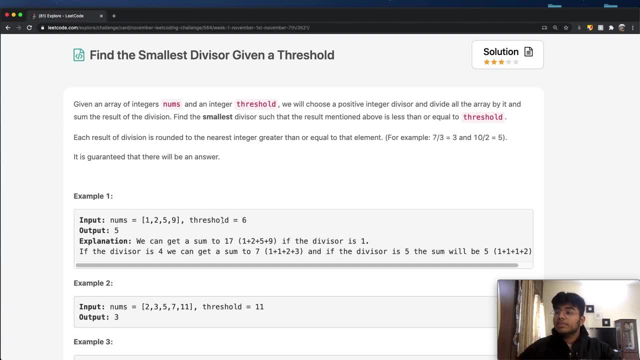 compare that with our threshold value. So after that we want to sum it up, So we're going to find the smallest divisor, such that the result mentioned above is less than or equal to the threshold. So in simple words, we want whatever value there is that is closest to the threshold. 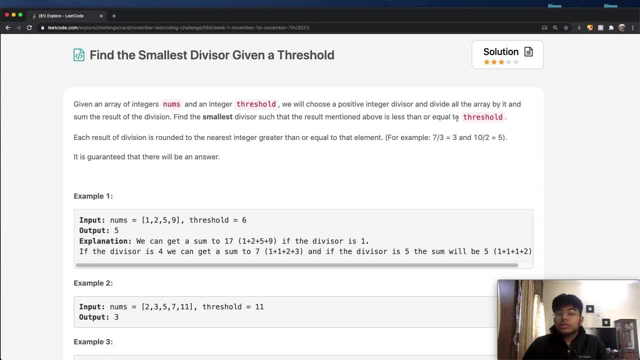 So ideally we want something which gets us exactly equal to the threshold, But if that's not the case, we want something which is closest to it, but it has to be smaller than our threshold. Okay, so each result of division is rounded to the nearest integer greater than or equal. 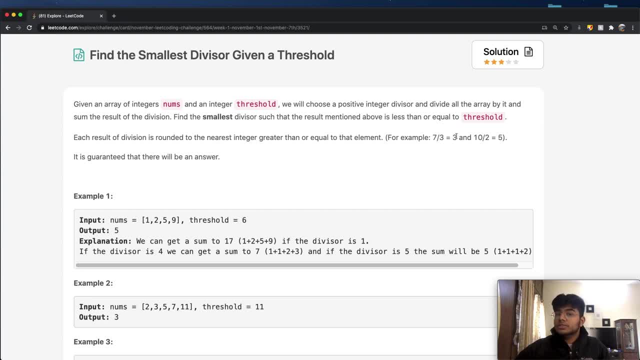 to the division. So, for example, seven divided by three is going to be equal to three. So we're basically going to round it up to the nearest integer value, and 10 by two equals five. Okay, so it is guaranteed that there will be an answer. So we don't need to worry about the fact where we don't have an answer. 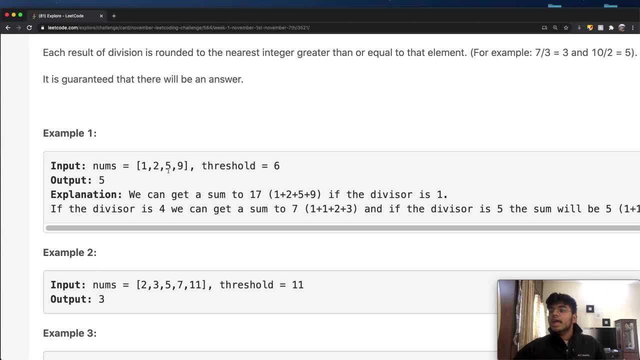 Alright, so let's just look at this question over here real quickly And the numbers we have is one, two, five and nine, So let's talk about the smallest divisor we can have. So the smallest divisor that we could possibly have is going to be the number one. So why? 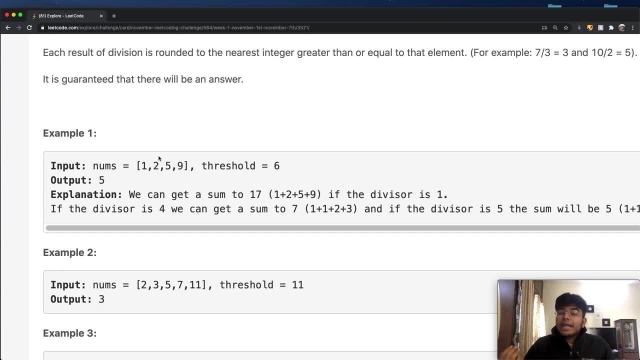 is the number one. So when you have the number one, what's going to happen? you divide each number by one, And when you divide something by one, it stays at the same value. So in this case, when you divide everything by one, it's still going to be the same as one, two, five and nine. 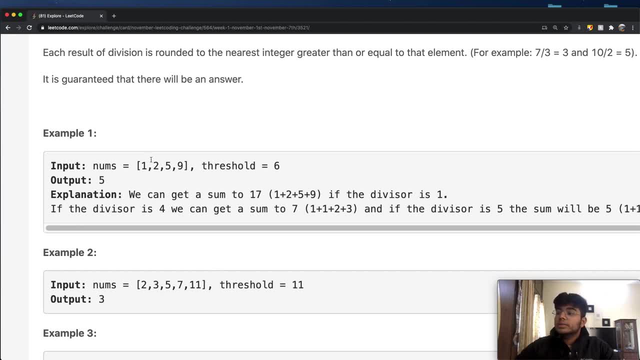 So our maximum value which we would get is going to be one plus two plus five plus nine, which gives us a value of 17.. So 17 is actually bigger than our threshold. So that means we want to look for a bigger divisor. And the reason we're looking for a bigger divisor is because bigger the 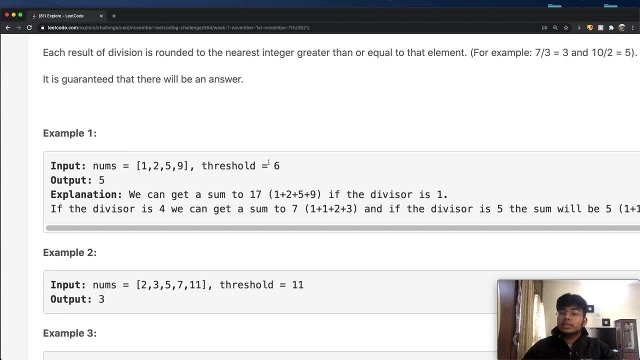 answer smaller our answer. So, for example, now let's say we go with a divisor of two. So in this case we'll do one divided by two and that gives us 0.5. But we're going to round it up to one. So 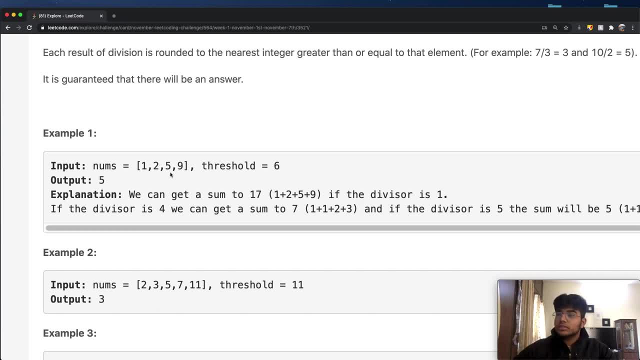 now we have one. now we're going to do two divided by two, which is also one. So now we have a total sum of two. then we have five divided by two, which would give us 2.5.. So we're going to round. 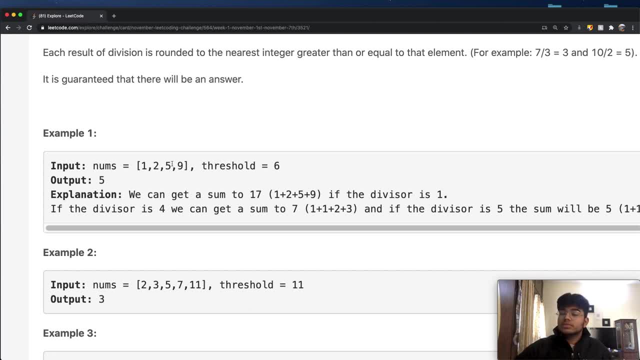 that up to three. So in this case we're going to have three plus two. So now we have a total of five. And finally, nine divided by two is going to be 4.5.. So we're going to round that up to five. 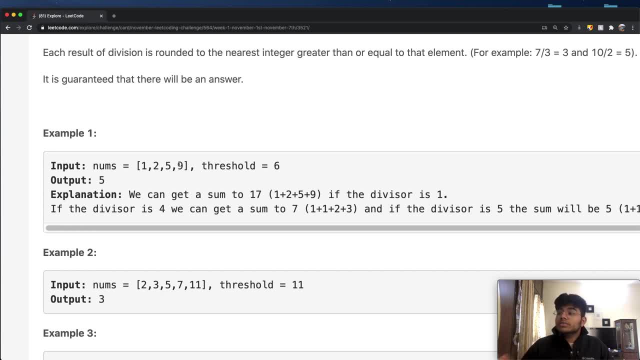 And now we've got an answer. So 10 is also greater than our threshold. So now we're going to change our divisor to three. So now we're going to get some value. then we're going to do four, and so on and so forth. But in this case 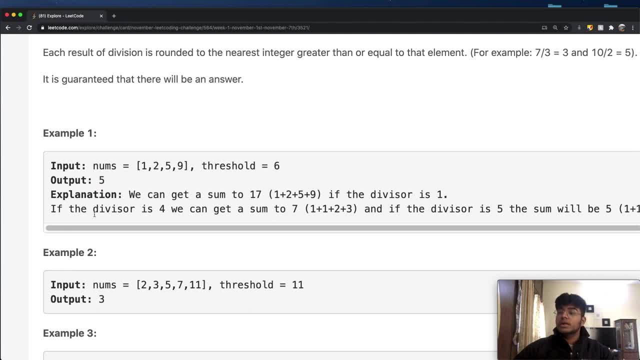 the correct answer is: when we get the value five, So let's just say we have a divisor of four. So when you have a divisor of four, we get a sum of seven, and seven is just right about the threshold. And now, when we use a divisor of five, the sum ends up becoming five. Okay, and that's the answer. 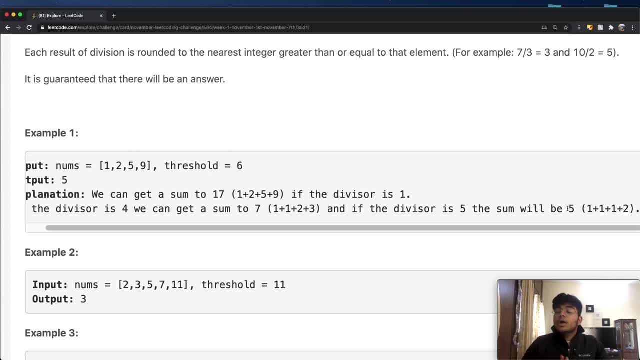 that we're going to end up outputting because that is closest to the threshold while still being smaller than it. So now let's kind of talk about how can we solve this question. So one thing we could do is we can go through all. 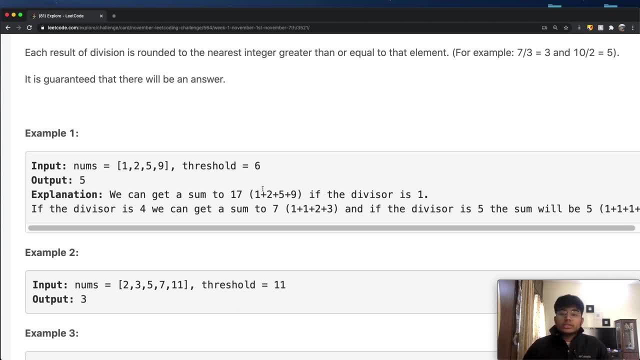 of the divisors possible and come up with the closest or best solution from that. But how exactly do we choose a solution? So what are the bounds to a possible solution? So the smallest value, like we talked about earlier, is going to be one. The smallest value is always one, And the biggest 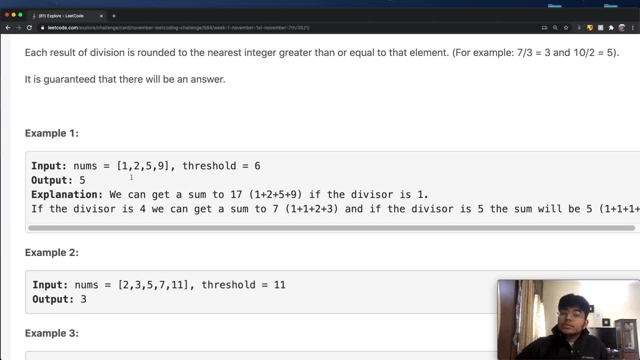 value of a divisor that we could possibly have is going to be whatever the maximum value is inside of numbers. So how does that make sense? So in this case, the maximum value is going to be the number nine. So in this case, when you divide everything by nine, so when you do one by nine, you're going 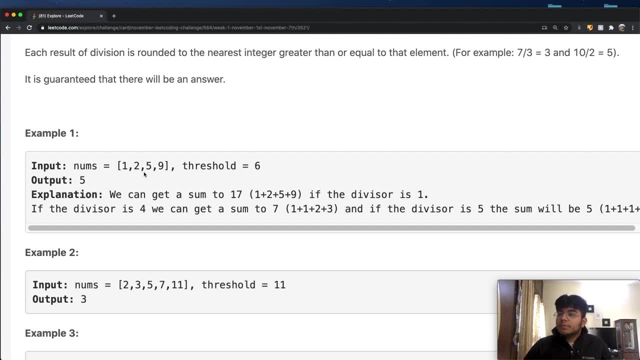 to get 0.something. Okay, but in that case what's gonna happen? that just rounds up back to one. So two divided by nine is after rounding. it gives us a value of one, same for five by nine, And in that case nine divided by nine is also going to be equal to one. So that is going to be our upper. 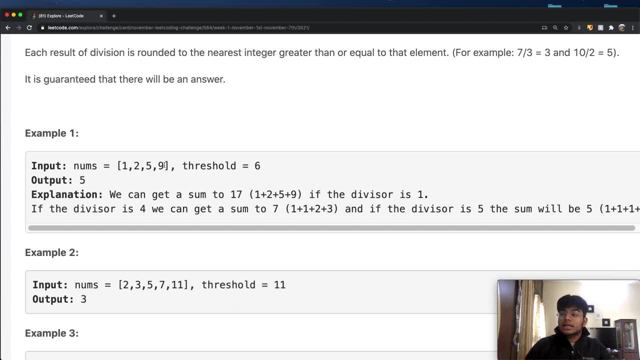 bound. the upper bound is going to be whatever the maximum number is inside of numbers, And when you divide everything by that number, you're going to get a value of one. So in this case, dividing everything by nine, our sum would be one plus one plus one plus one, which is well for Okay. 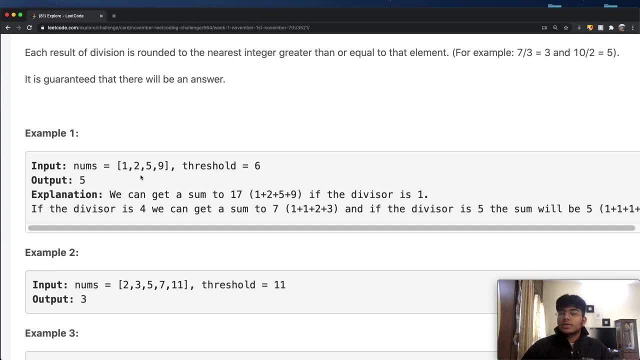 so yeah, that's going to be our upper bound value. Okay, so you can kind of see that there is a boundary right between one to nine. So to make this a little bit more efficient, instead of looking for each and every value, so 123456789.. Instead of doing that, we can actually 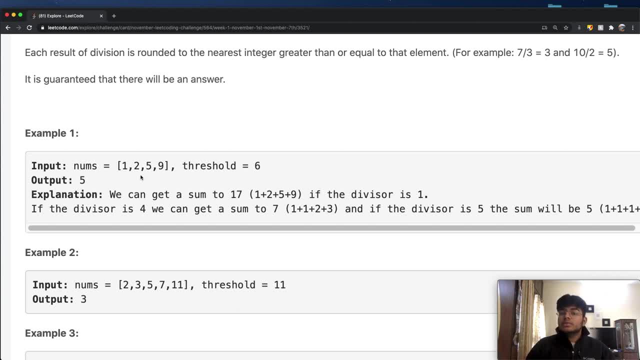 selectively choose which values you want to find. So let's say we start off at the very middle. So in this case let's say we start off with five, And that actually ends up giving us our answer. But let's just kind of generalize it. So we're going to start off at the middle of our boundary. 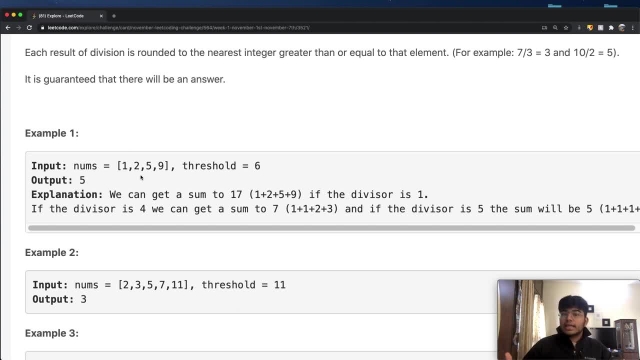 Now, in this case, we're going to get some sort of answer, And if that answer is greater than our threshold, then in that case we want to look for a smaller sum, And when that happens, what we're going to do is we're going to move our left or our lower point bound value. 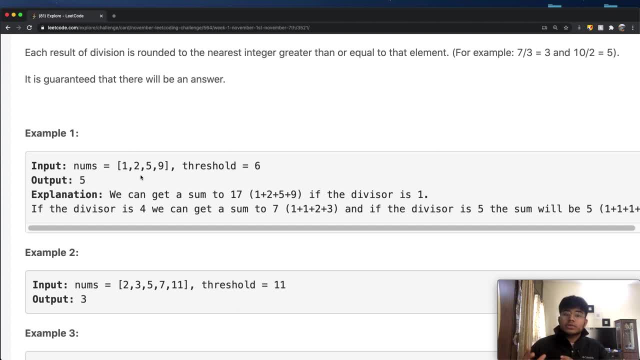 to the right, And the reason we're doing that is because when the threshold, or the value that we end up outputting, is bigger than the threshold, that means that we have a smaller divisor and we want a bigger divisor. And if the case is the other way around, so let's say the value we've 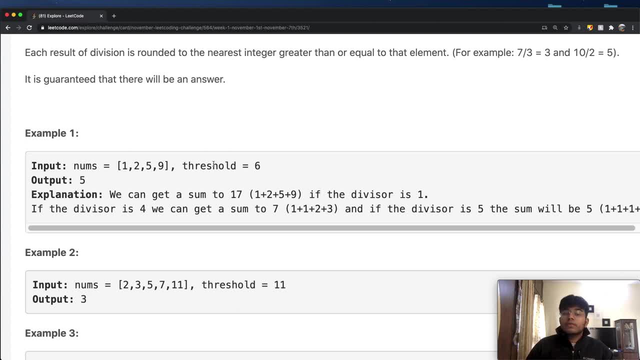 got is too small, then in that case that means we're looking for a smaller divisor And in that case what's going to happen is we're going to move our right pointer to the left, So we only look at the smaller value. So you can kind of understand what we're really doing. 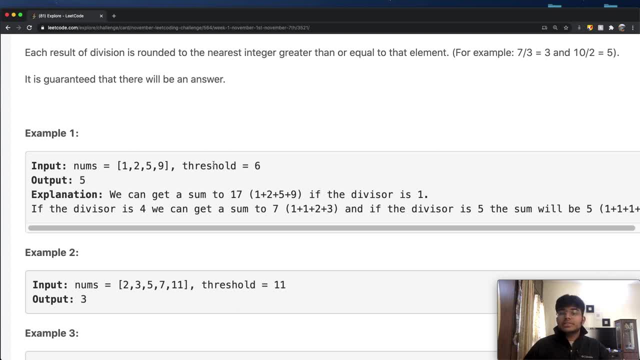 is a binary search, because we have a sorted list of numbers and we're just going to try to search for the best possible divisor. So now all we need to do is kind of implement it and see how it actually works. Alright, so let's start off by actually defining our two pointers. So we're 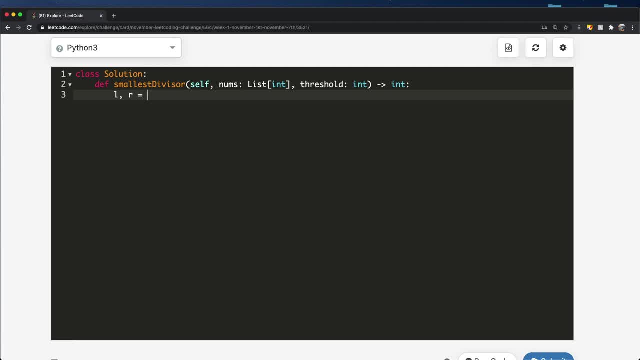 going to have a left pointer and we're going to have a right pointer. So the left pointer is going to be the lower bound value. So the lower bound value here is going to be one and the upper bound value, like I said, is going to be the maximum number inside of num. Okay, so we have our two. 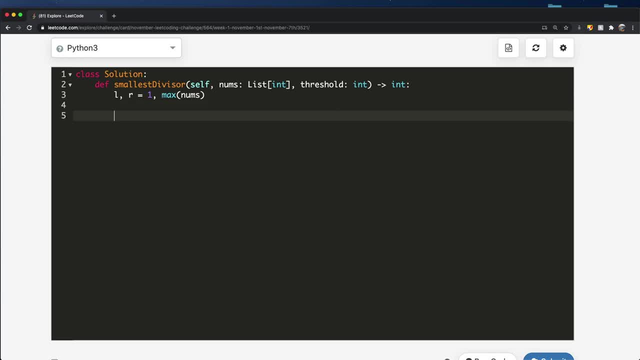 boundaries now. So now we're going to go inside of a while loop. So what we're going to be doing over here is we're going to be going into this while loop as long as left is less than or equal to our right bug. The second, the left value becomes greater than our right value. That 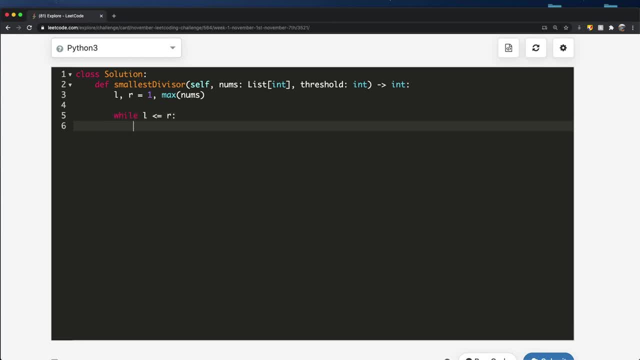 means that we have found our answer and we can stop it. So the first thing that we want to do over here is we actually want to find out what's the middle value. So, to find out what the middle value is, what we're going to do is we're going to 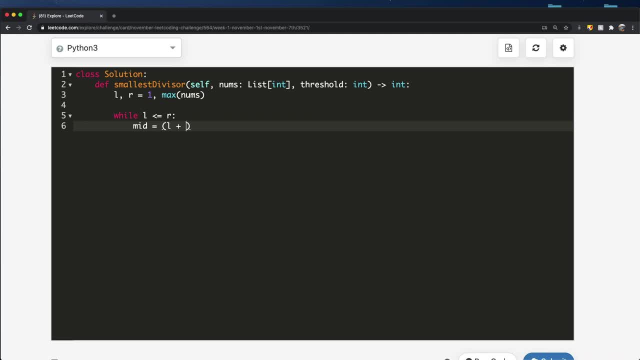 take our left pointer for the left boundary. we're going to add that with our right boundary and we're going to divide it by two. But one thing that we want to do over here is we're actually going to end up doing integer division, because we want an integer value and we don't want a. 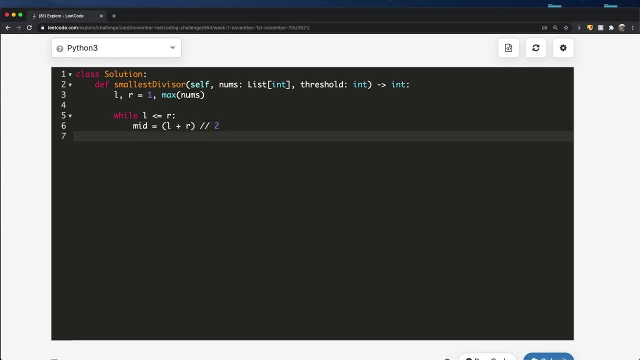 decimal. Okay, so now we have an integer value which we are considering to be our midpoint. So now, whatever the midpoint stands for, so the mid value that we have over here, it's nothing else but the middle value. So we're going to take our left pointer and we're going to divide it by two. 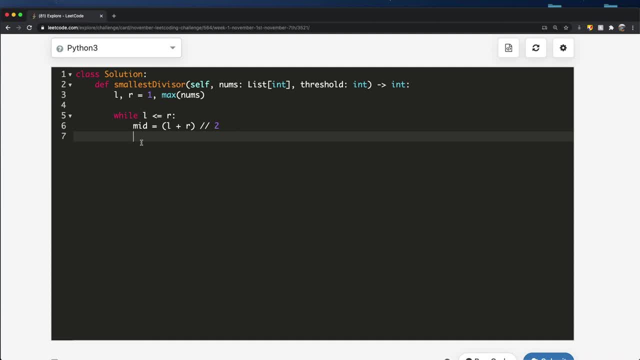 The divisor, but we didn't get an answer yet. So now we actually want to come up with an answer. So how exactly do we come up with an answer? So to actually come up with the answer, first, we divide each of the things inside of our array num by the mid value. 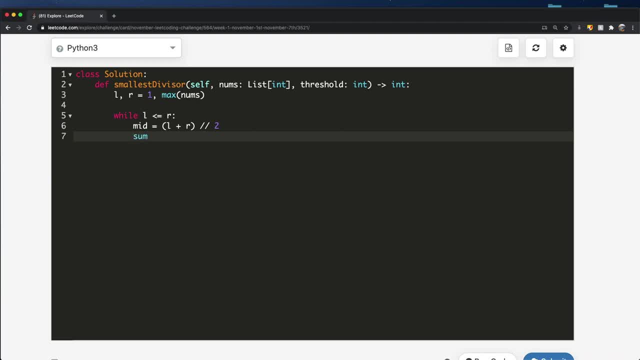 and then we want to add them all up. So let's see how we can do that. So we're going to be using sum, And over here we'll be using comprehension to actually get that done. So what we're going to be doing is we're going to take a number and we'll so the 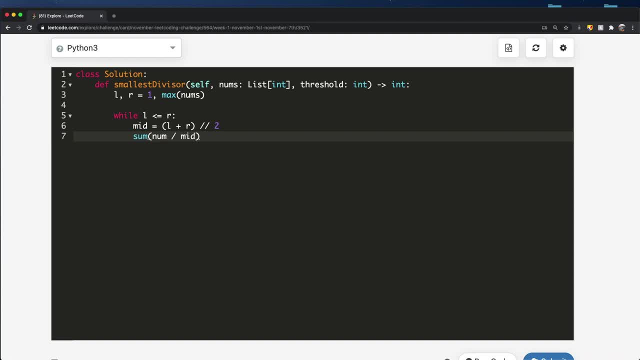 num and we're going to divide our number by the mid value. So now, how do we get our numbers? So to get our number, we'll do for num and we're going to get it from our nums array. Okay, so one thing that is wrong over here- or not wrong, but we need to change- is when you do num divided. 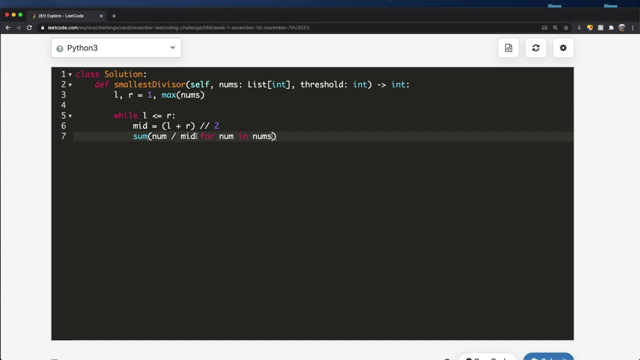 by mid. we might actually end up with a decimal value, But we're only looking for integer values And even if it does end up becoming a decimal value, we're going to round it up. So, since we're going to be rounding it up, we're going to round it up by a decimal value. So, since we're going to